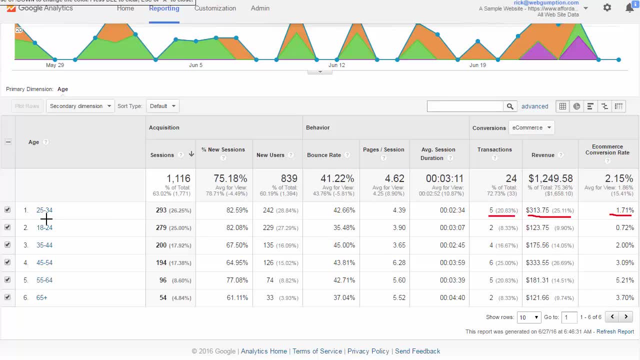 Now what's interesting is, if we compare this age group- our most common- to this age group, we have the 55-64 age range, which makes up a very small portion of our traffic- less than 9%- but at the same time yielded about the same number of transactions- less revenue. 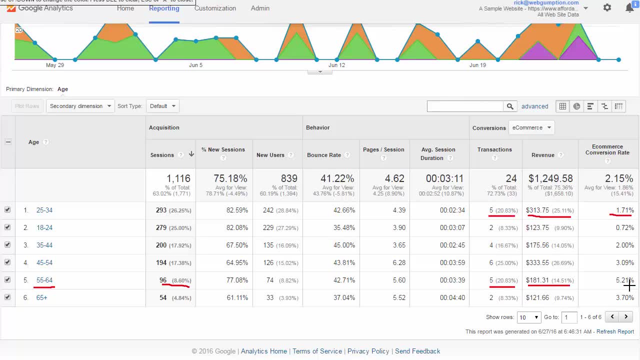 but showing an e-commerce conversion rate that's about 5.2%. So it's roughly three times higher as far as the conversion rate goes. So if we're thinking analytically at this report, you know it's nice to know what the different age groups are. 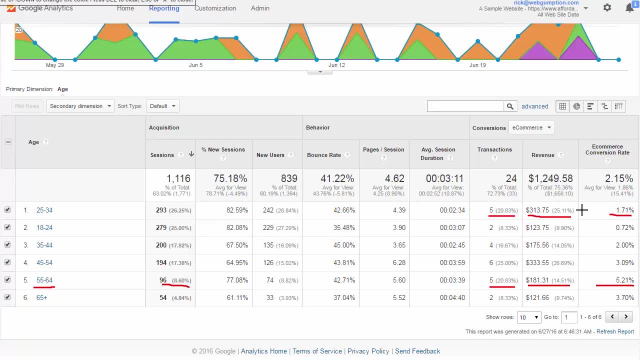 but how we can act on this is: we're going to look at the conversion rate. Well, hey, if this age group 55-64 converts at a much better rate, should our advertising reflect that. So should we run Facebook ads, for example, to individuals in that age group. 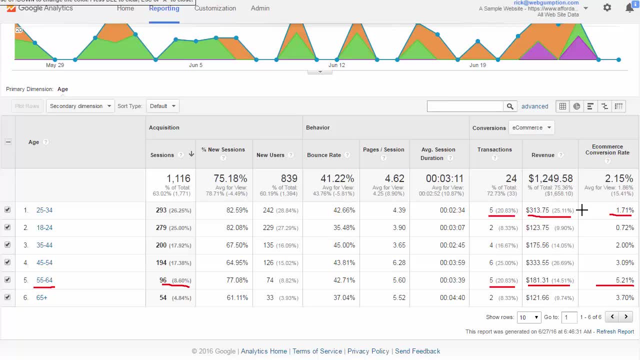 Or should our display advertising target that age range a lot better? These are some of the things we want to consider with the age report: looking for those outliers and finding marketing opportunities. Demographics, gender report. So, demographic gender report: we're going to look at that.